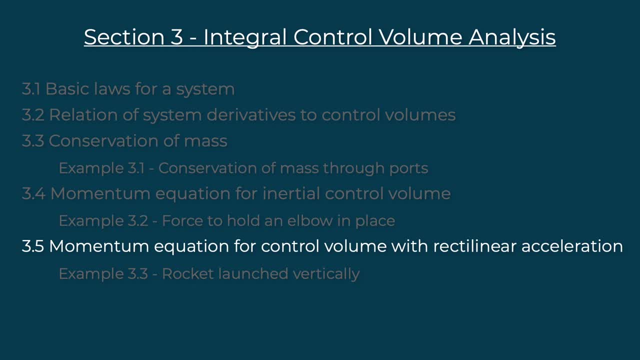 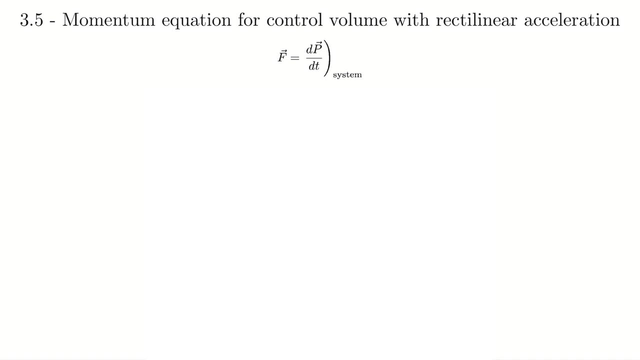 a control volume where the control volume itself is accelerating. Okay, so we can think of the classic example here being the rocket that's blasting off. Okay, so we'll just look at one term here in this title that we might not be familiar with: rectilinear- Like that word makes me think. if I was like at a doctor's appointment and my doctor started saying, like rectilinear, that I would like be concerned about that. But anyways, what does it really mean? So rectilinear means we're moving in straight lines, And the key aspect of that is that there's no like rotational component of our 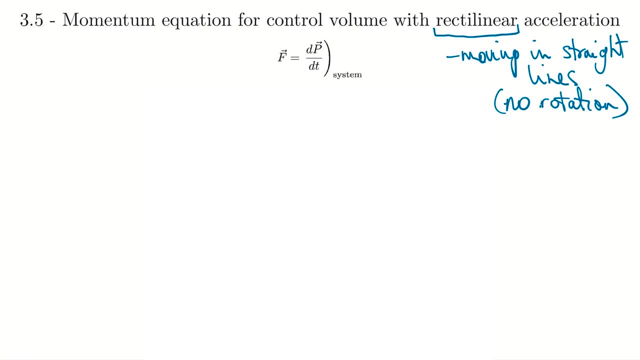 acceleration. Okay. so we know, in this one we're going to be building upon what we did in the last subsection, when we had force balances of control volumes that were not accelerating. So again, we're starting here with Newton's second law, which we've seen a few times now. right, And we remember that that's in reference to a system. Okay, now I'm going to walk through this breakdown, but I'm not going to do again, I'm not going to do a detailed derivation, just going to walk through and we're going to discuss how we include the acceleration into our equation. So the key here is to really look at two different things we're going to be looking at. 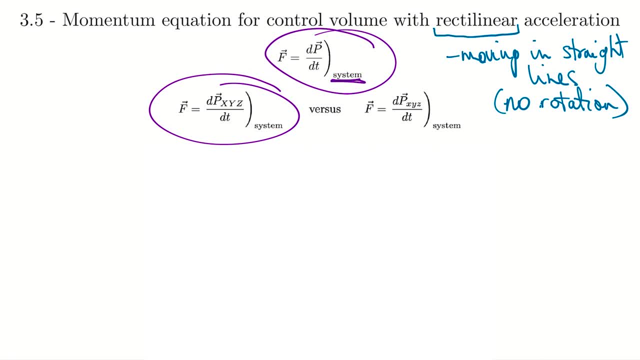 our relative reference frame. And so on the left, with the capital XYZ, we remember, now that's in reference to the ground, So we have that as, like, our stationary reference point when we looked at control volumes moving with a constant velocity. So same thing here. And when we use lowercase XYZ, now that's the reference frame, that is the control volume itself. So that's relative to the control volume itself, which now is accelerating. Okay, now Newton's second law is based on the one on the left, So our force is equal to the rate of change of linear momentum. 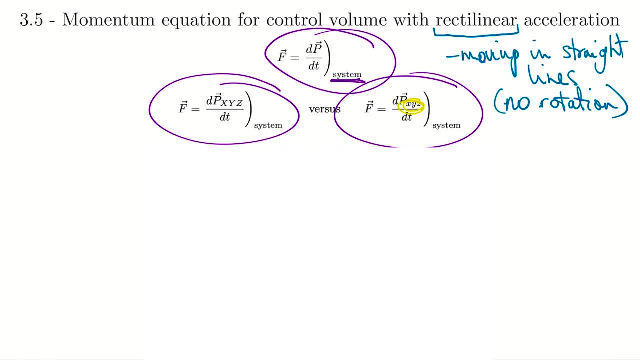 that's relative to our inertial reference frame right, the not accelerating one, but the one on the right relative to the control volume. that's the one we're going to want to use to calculate this right, Because, for example, if we think about the rocket and we have fluid, you know, crossing the boundaries, right, so shooting at the bottom of the rocket, all that information is going to be relative to the control volume itself. So the easiest way to go about this is just to account for the fact that the reference frame is accelerating. So instead of saying the force is just the rate of change of the linear momentum, we'd have to then add a component. 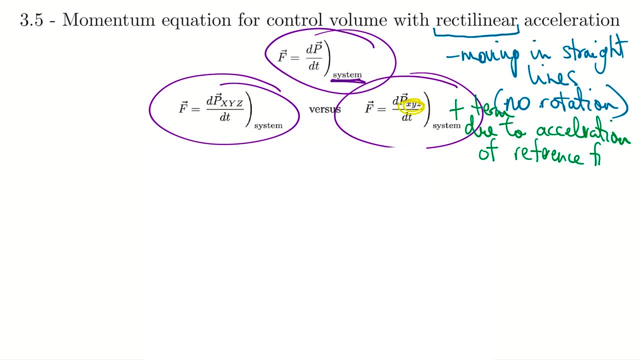 onto that. that accounts for the acceleration of the reference frame. Okay, we see how we do that mathematically. on the line below we'll move it over to the left And we'll see now the force minus the mass of our system times the acceleration of the reference frame, that equals to the rate of change of linear momentum. So that's like a rewrite there of Newton's second law, where we now directly factoring in the fact that our reference frame is accelerating. So the RF is reference frame, And so we know what we can do again when we have this integral relative to our mass or our system is. we've done this trick a few times. we were 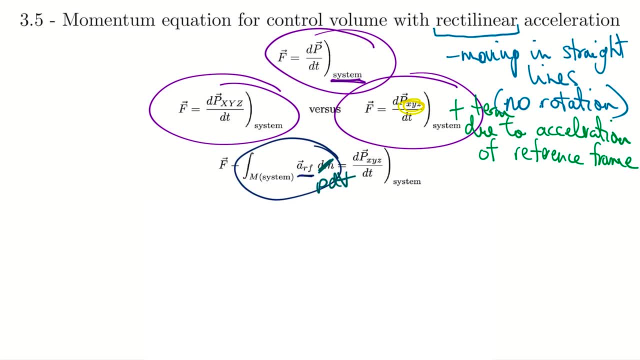 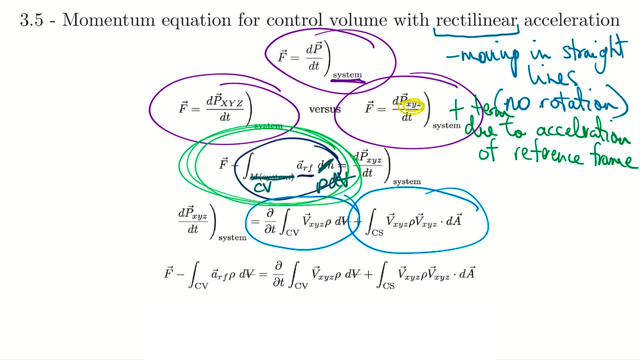 go ahead and we're going to plug in what we had on this line, right, instead of just force, it's the force. And then we also have to consider the acceleration of the reference frame. We put that here, Okay, and now it's a full equation And we can see. really, the only difference in this is that we've added in this single term here that accounts for the fact that our reference frame is accelerating, And by reference frame, as a reminder, we mean the control volume itself is accelerating, right, So we'll do an example after this, So we can really see this. but that would be things like a rocket, where you draw the control volume around the rocket itself. So then, one more simplification on that. 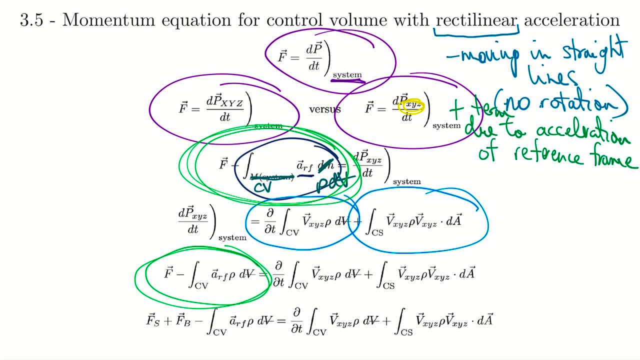 line below. we know our external forces are going to be the surface forces and the body forces. we've seen that breakdown before. we can break all the forces out into surface and body forces. so in the line below that's just kind of the complete form there. okay, so we box that one because we can use. 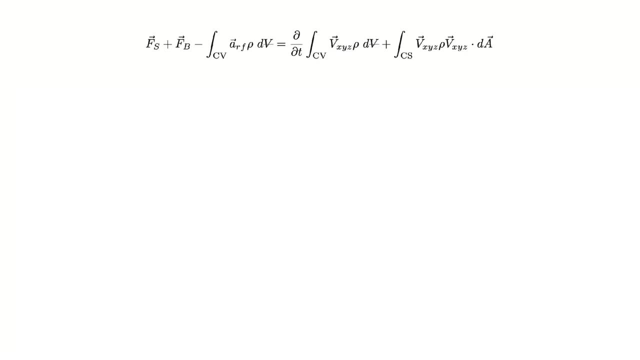 that one. i'll throw that on a fresh slide here, because most often what we're going to be using is the component form of this right, as we did for the inertial control volumes. so i've broken it out into the component form here and again we can see that there's just this one term that's different. 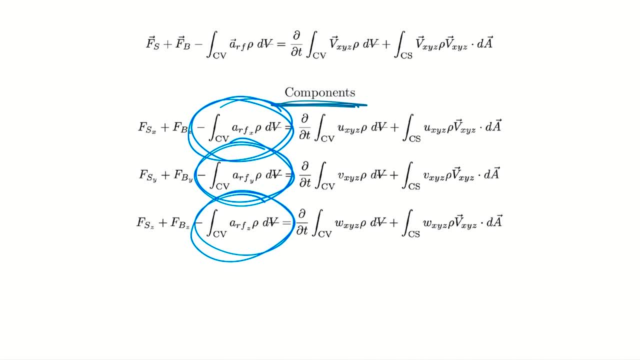 in each of these. that's the only difference from the inertial frames, and then the term on the far right. so i'll circle them, these ones here, where we're accounting for the linear momentum that's crossing the boundary, if we have what's inside the integral here, if that's not changing over the area. 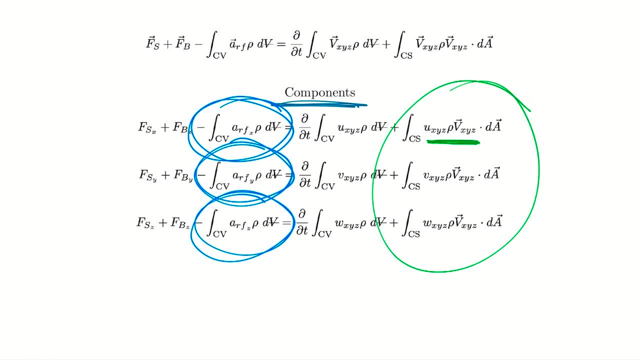 so we have a uniform velocity or an average velocity, which again is very common. remember that v dot da is just q or volumetric flow rate. we might have that value or we might have rho times v dot da, which together is our mass flow rate, very common in these questions, as we'll see from the 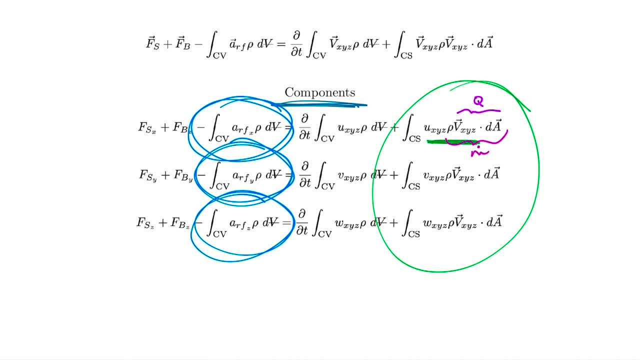 examples, to have either of those, but we're going to go ahead and do that and we're going to go ahead and do that and we're going to go ahead and do that. so in the case where we would have the uniform or the average velocity, we don't have to integrate and we remember we can replace that. then we 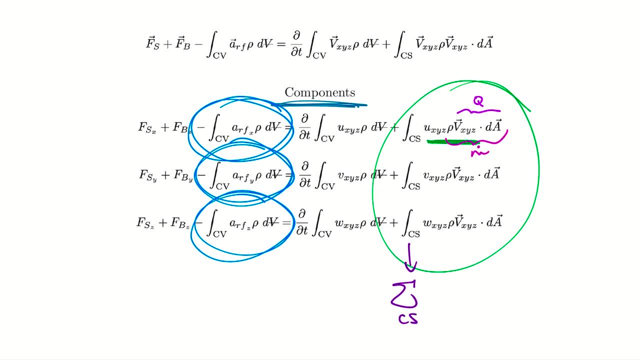 replace that integral with a summation instead- and i haven't written them all out again because they're just the same thing. we've seen this before, but remember that can be replaced with a summation for the case where we have uniform velocity, and that'll be the one we use the most often in the 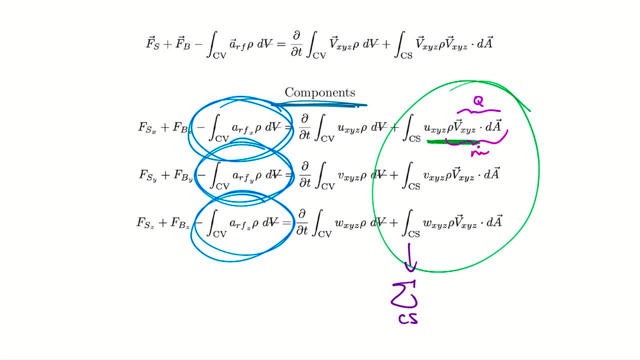 examples. and just an important note about that term circled in green there. that is what we commonly refer to as thrust. okay, so that's the force that's generated because we have a fluid moving across our control volume boundary. so the idea there is: you can shoot this fluid out. 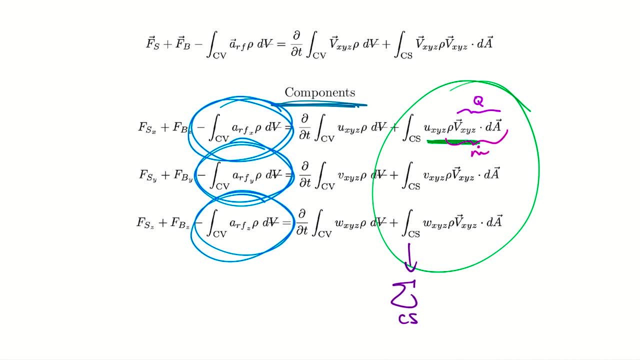 from the object and that generates a force that we call thrust, and we've seen that driving our airplane turbines, we see that driving rockets. that's the force that drives the rockets. so i like the connection there to think of that term as like our thrust term. okay, so that's really. 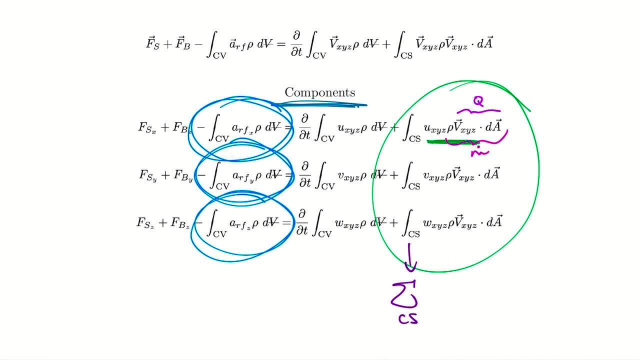 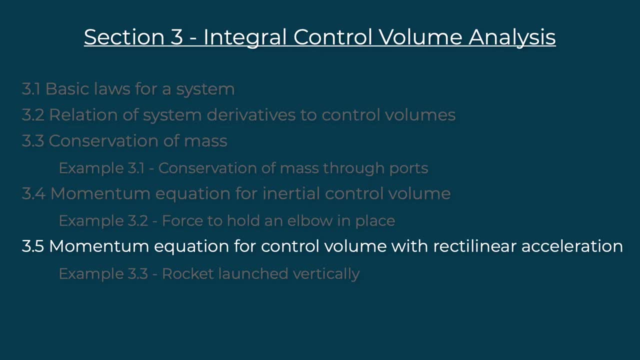 all for this. there was just the one term that's different. uh, now i think again. i think it's really nice to do examples so we can really see this. so a quick summary on this one: was we just, in this case, force balances for control volumes where the control volume itself is accelerating? classic? 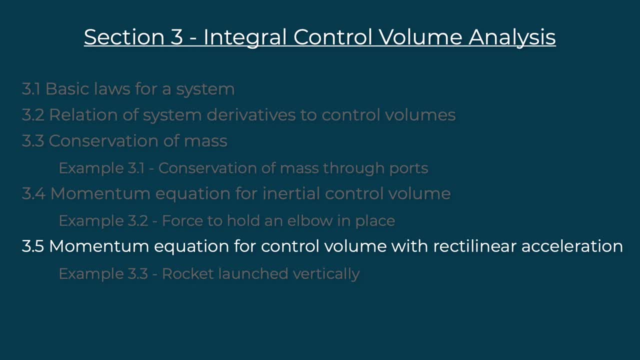 example, there would be like the rocket: rockets your control volume and as it blasts off it accelerates upwards, and then we determine which equations to use. really, the only difference from the inertial frames- the ones that were not accelerating- was we had to just add one more term.